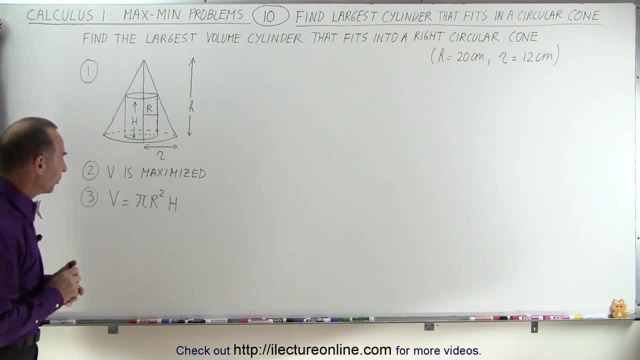 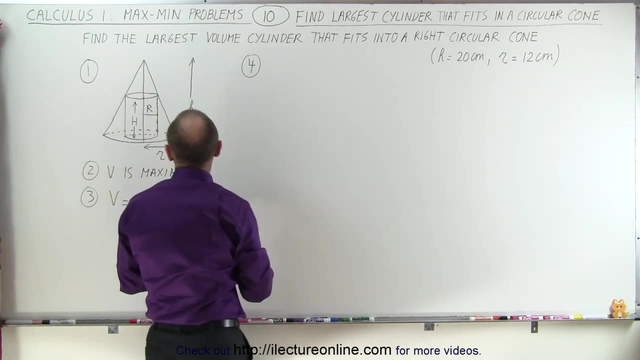 which means that the volume is maximized. That means we're going to have to eliminate one of those variables. For that we're going to need a constraint. How do we come up with a relationship between R and H so that it fits inside that right circular cone? 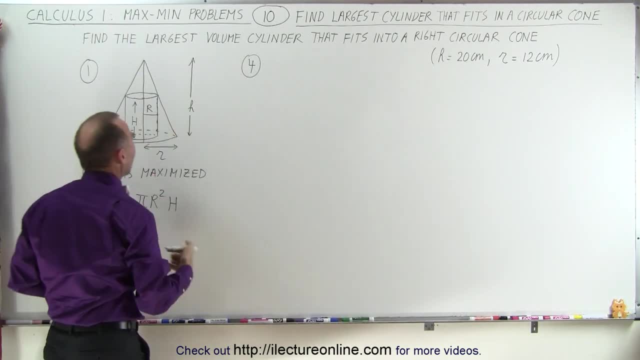 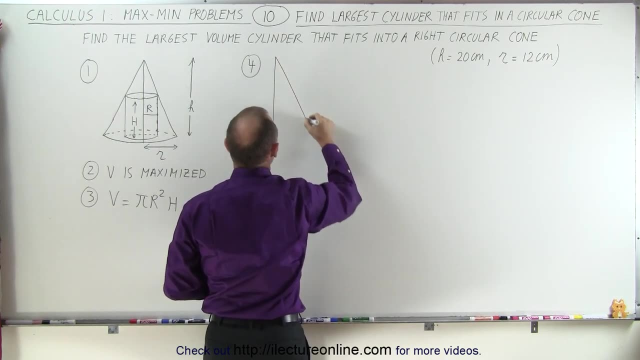 Now, if we think about taking a cross-section of that and taking just the right side of it, it can look like this: So this would be a cross-section of the right circular cone and this would be a cross-section of the cylinder. 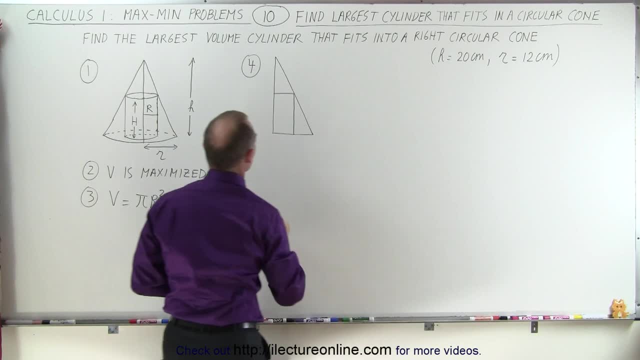 that fits inside the right circular cone, so that we have the height of the cylinder in this direction and the radius of the cylinder in this direction Also, we can come up with an equation for this line right here. That would be the edge of the right circular cone. 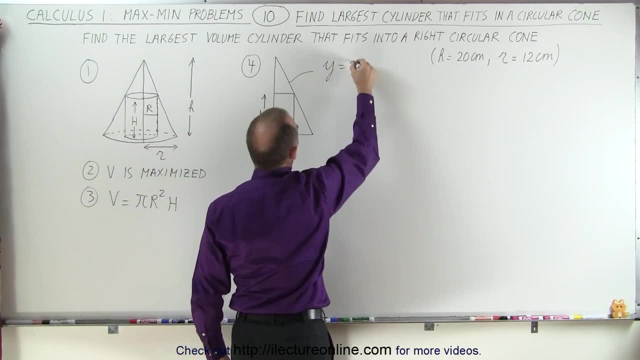 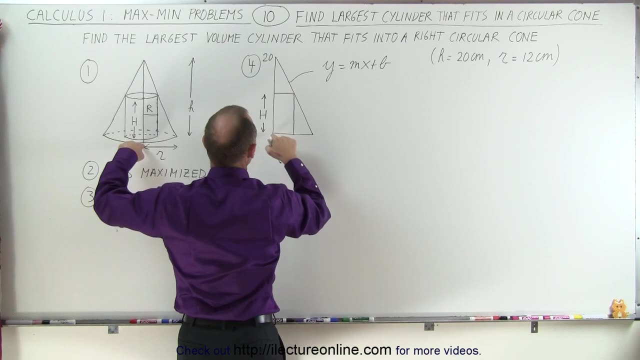 We think of it in terms of y equals mx plus b. Notice the intercept will occur at 20, because if we put the origin right at the middle, right here, we know that the height of the right circular cone is 20, and the radius of this is 12.. 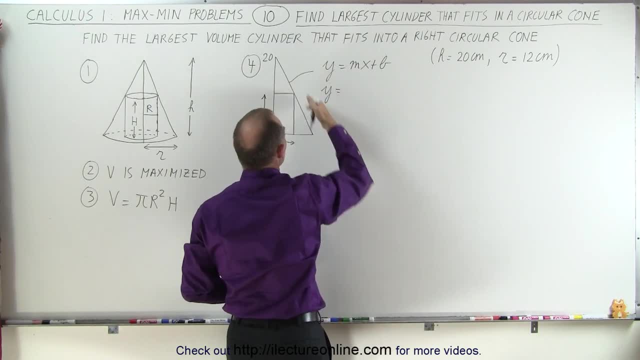 So we can say that y is equal to the slope. That would be a drop of 20 and a run of 12.. That would be minus 20 over 12x, plus the intercept which is at 20.. And, of course, simplifying that. 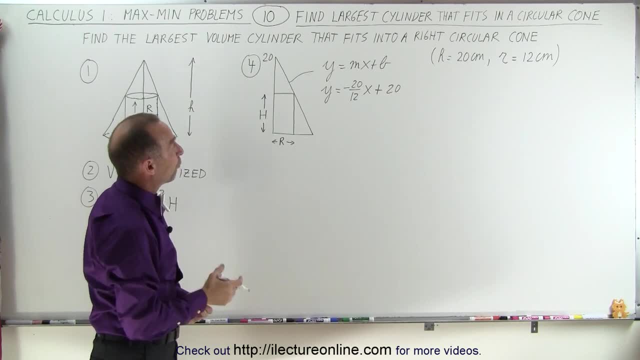 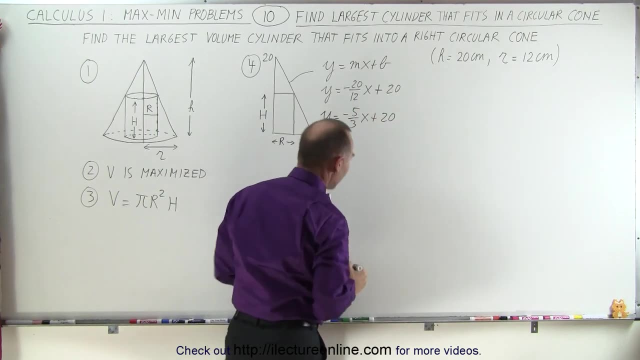 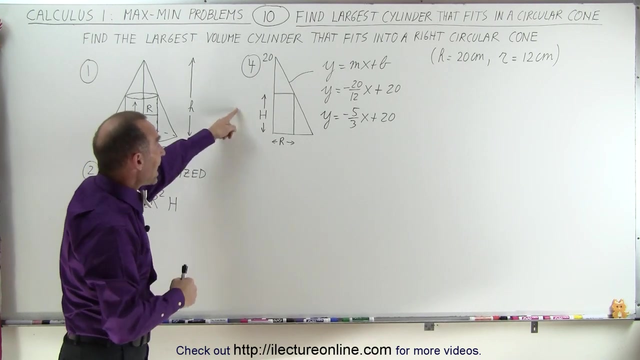 we can divide both the top and the bottom by, It looks like 4, so this becomes: y equals minus 5 over 3x plus 20.. Now it turns out that we can relate y and x to h and r, because they will have the same proportions. 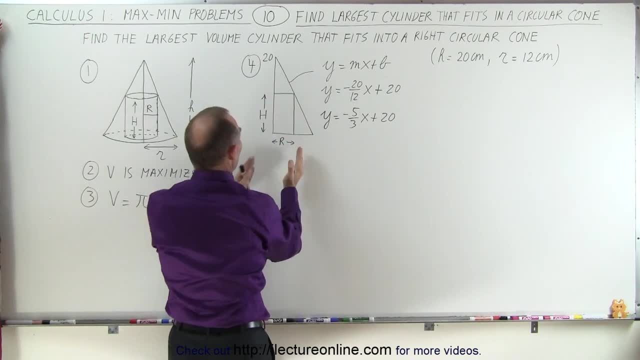 r would be the value for x and h would be the value for y. As x becomes smaller, y becomes larger. Therefore, as r becomes smaller, h becomes smaller or h becomes larger, I should say, So y can represent h. 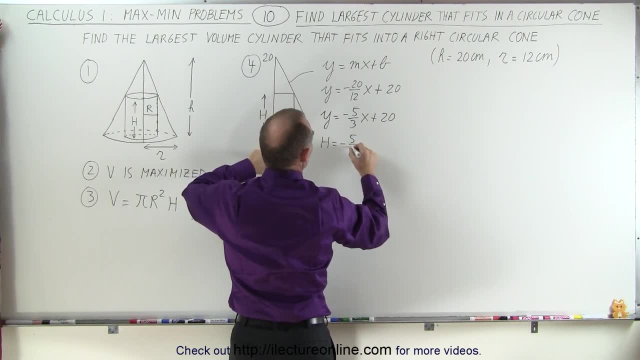 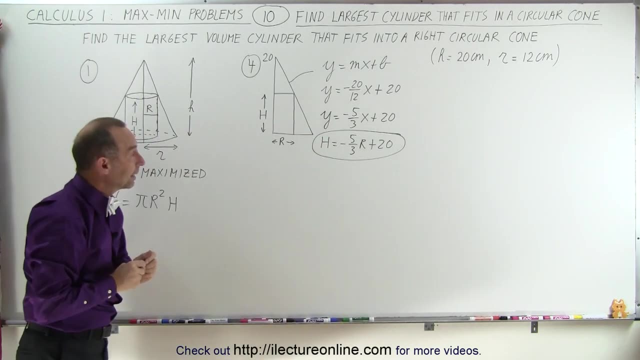 and x represents r. So this is minus 5 over 3r, plus 20, and now we have our constraint, or our relationship between the height and the radius of the cylinder. Once we have that, we can plug that in here. 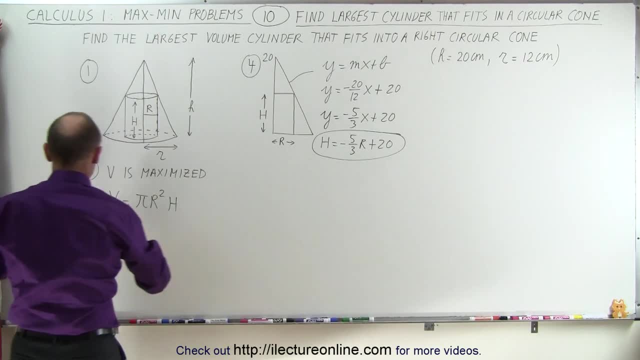 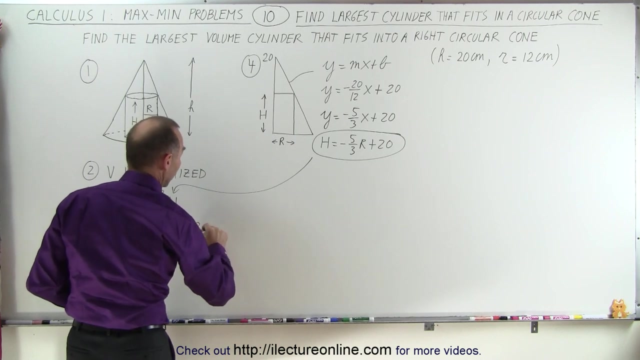 to limit one of the variables, and that's step number 5.. So now we can go ahead and take this, plug it in here and now we have: volume is equal to pi r squared times. instead of h we can write minus 5 over 3r plus 20.. 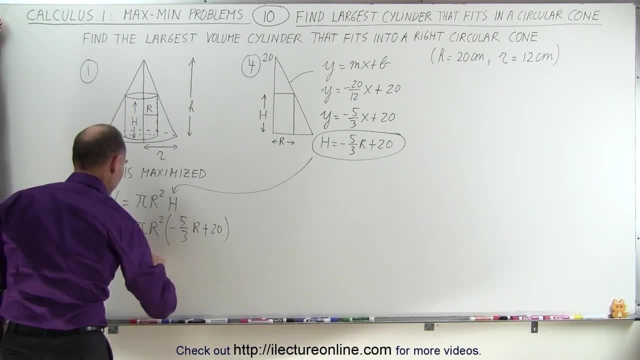 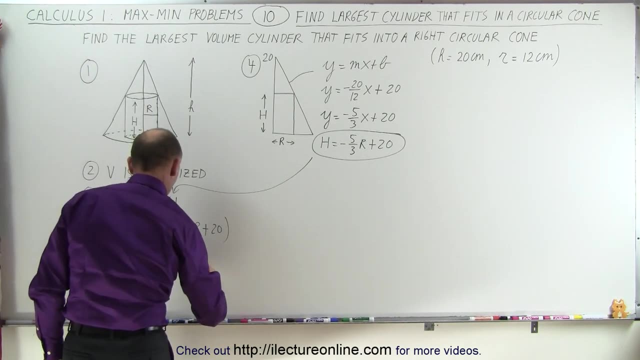 Of course, multiplying this out we get the volume is equal to minus 5 over 3 pi r cubed and plus 20 pi r squared. Now we have an equation for the volume, the item that we're trying to in this case. 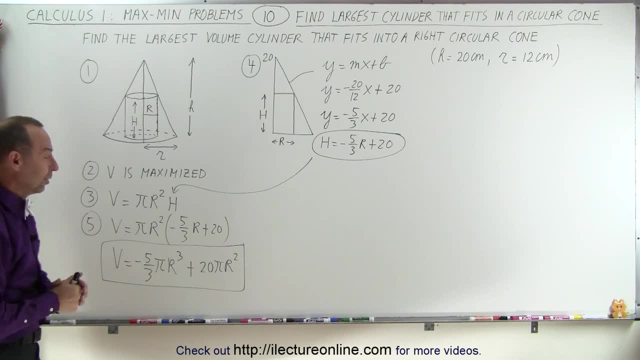 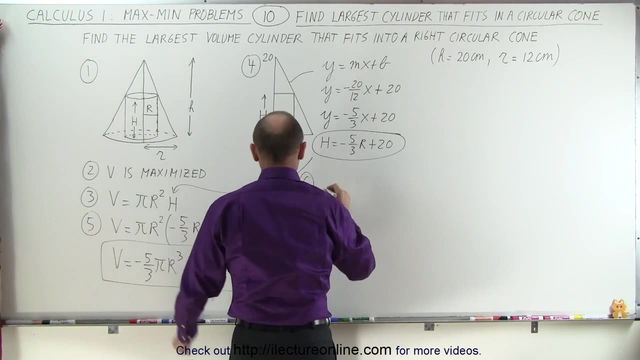 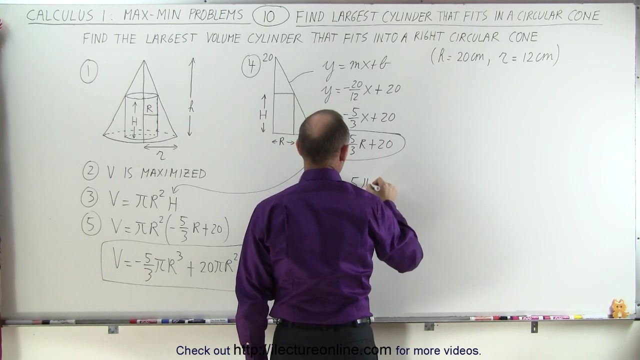 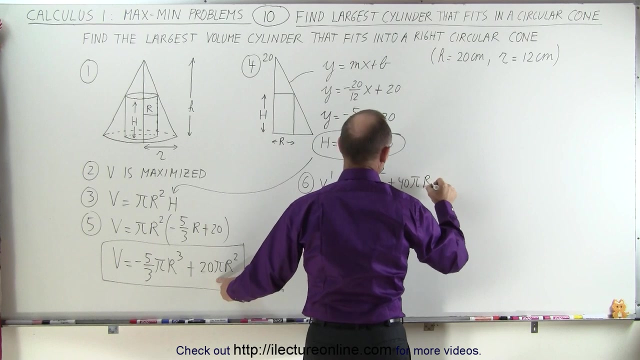 maximize in terms of only one of the unknowns. So the next step is to take the derivative and set that derivative equal to zero. We get v. prime is equal. to bring that down, we get minus 5 pi r squared. and here we get plus 40 pi r. 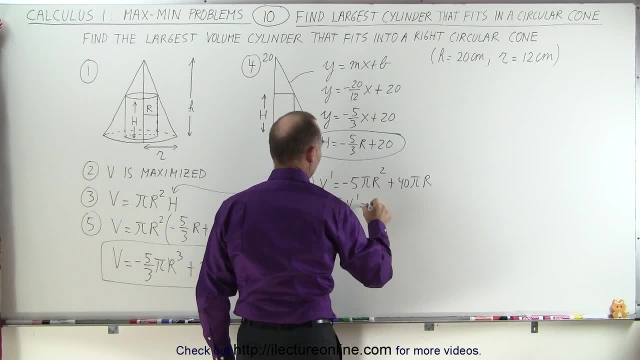 and now we're going to set v prime equal to zero. And again, the reason why we do that is because we're trying to find the maximum value. In this case, we're trying to find the maximum value, So we get: zero is equal to. 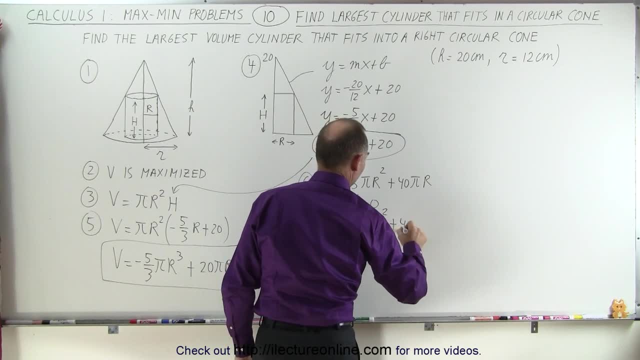 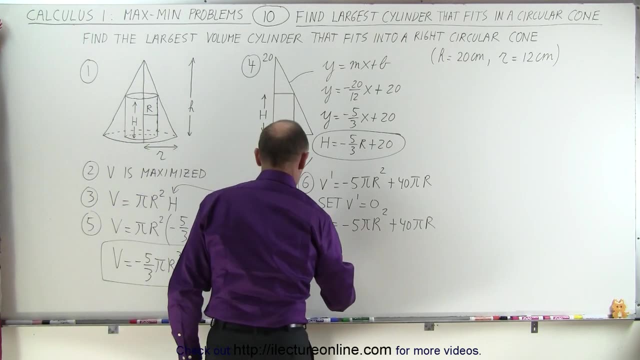 minus 5 pi r, squared plus 40 pi r. And now we're going to solve that. for the unknown variable r, First of all, you can see that we can divide both sides by 5 and both sides by pi, It becomes zero is equal to. 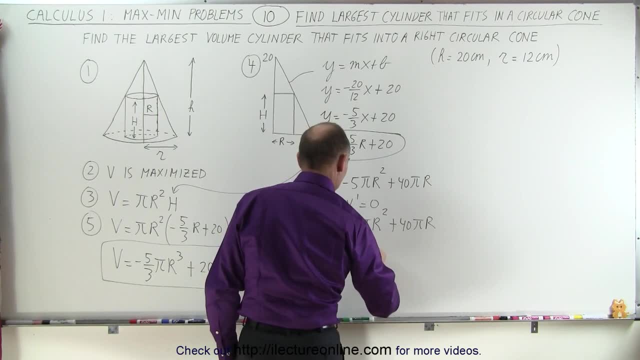 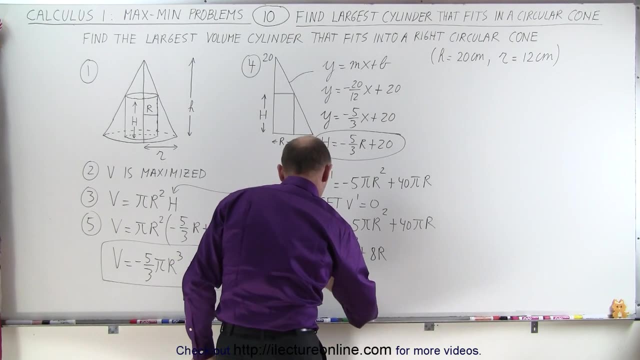 well, we still have a minus. so it's minus r squared plus 8r. So moving that to the other side, we get r squared is equal to 8r. and dividing both sides of the equation by r, we get r is equal to 8.. 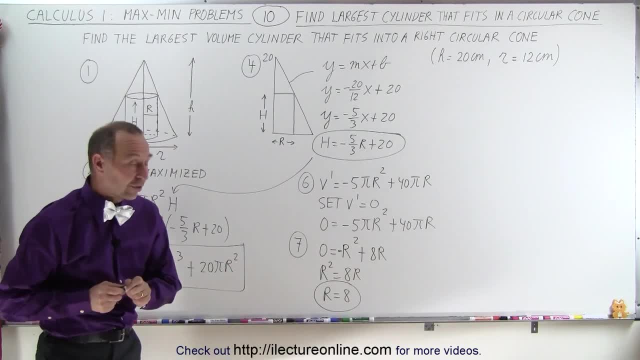 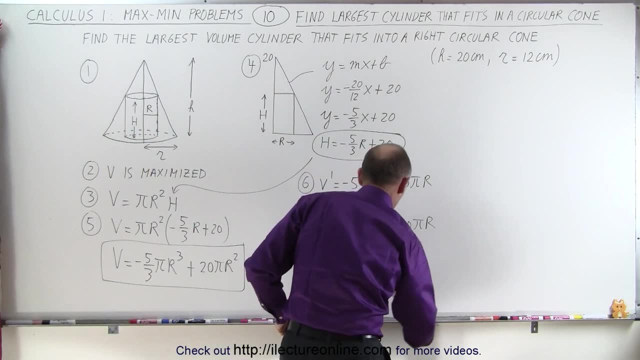 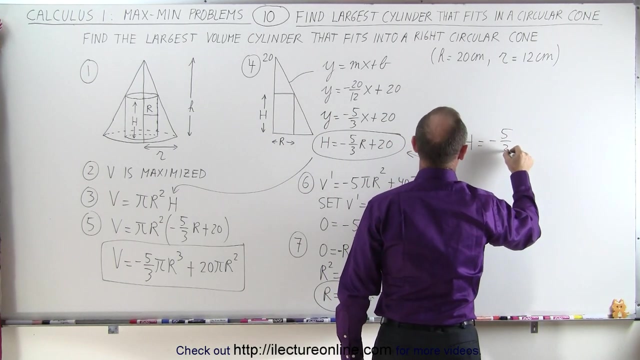 That tells us one of the two unknowns: the radius of the cylinder must equal 8.. Now we need to find the height of the cylinder. so we plug this value back into the constraint equation And that tells us that the height is equal to minus 5 over 3 times the radius. 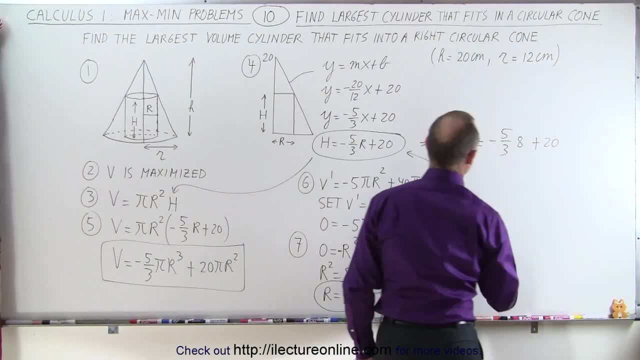 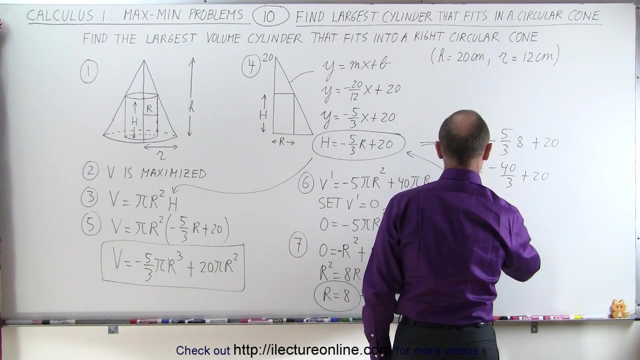 which is 8, plus 20.. So the height is equal to. that would be minus 40 over 3 plus 20.. Hmm, minus 40 over 3, that would be minus 13 and a third. so h is equal to. 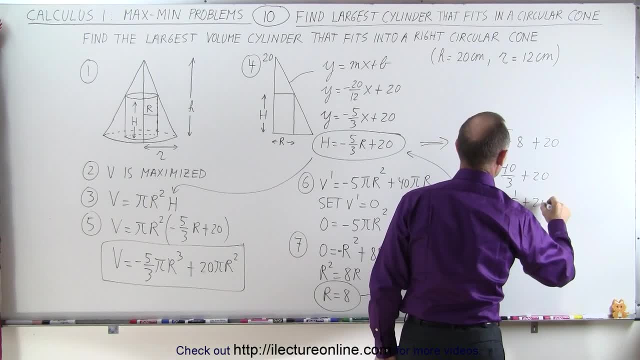 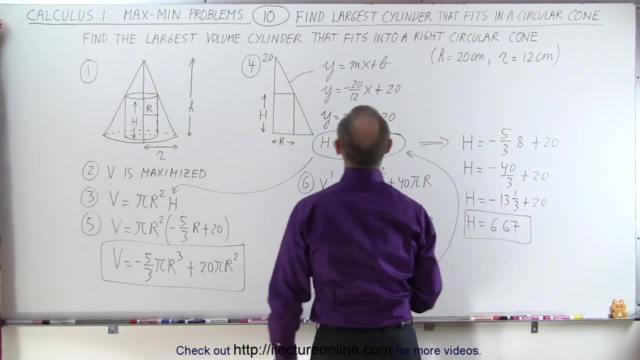 minus 13 and a third plus 20, which means that the height is equal to 6.67.. Of course, the units do we have some units, We have centimeters. of course the units then would be 8 centimeters for the radius. 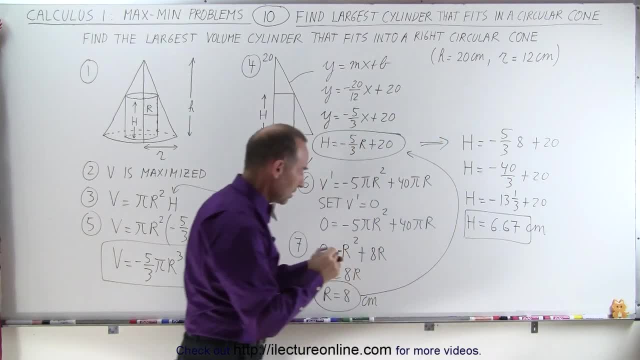 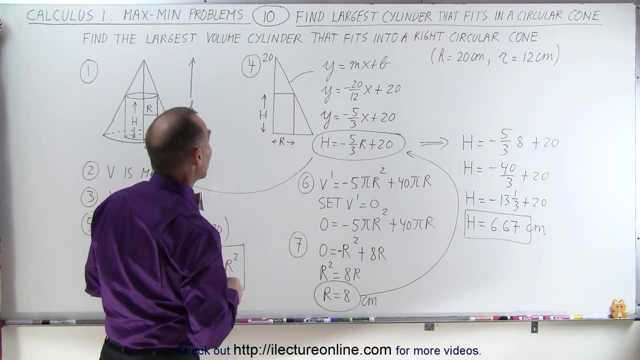 and 6.67 centimeters for the height. Now we can do a quick check. We can see if that indeed gives us a reasonable value for the volume. We can say that the volume of the right, the right cylinder. so we're going to do a quick check. 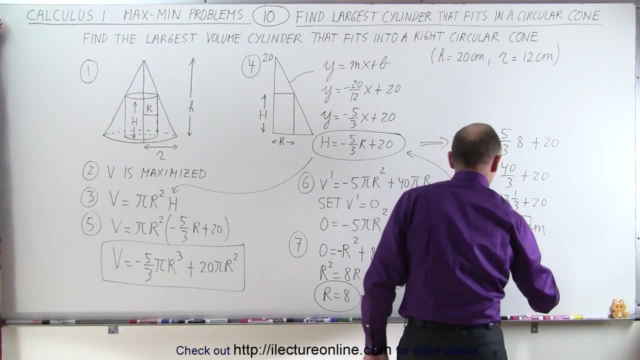 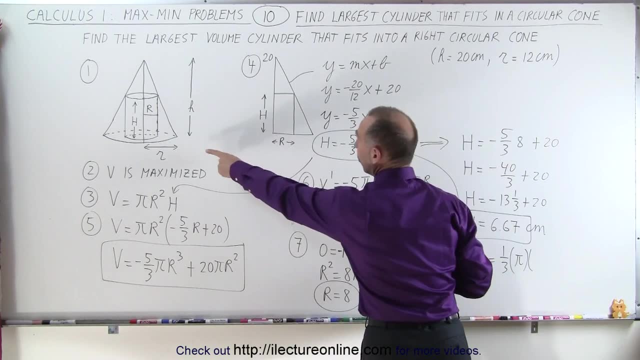 The volume of the- not the cylinder, but of the cone- is equal to one third the base, the area of the base, which would be pi times the radius squared. in this case the radius is 12, so that would be 12 squared. 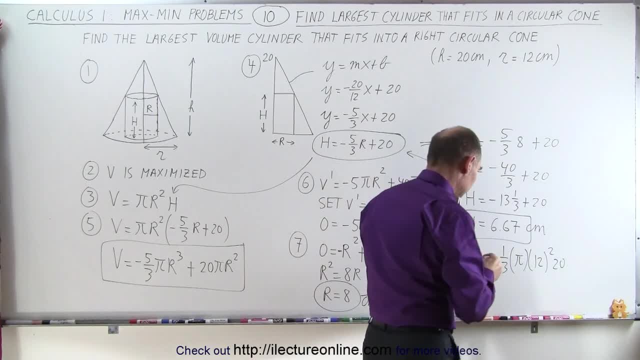 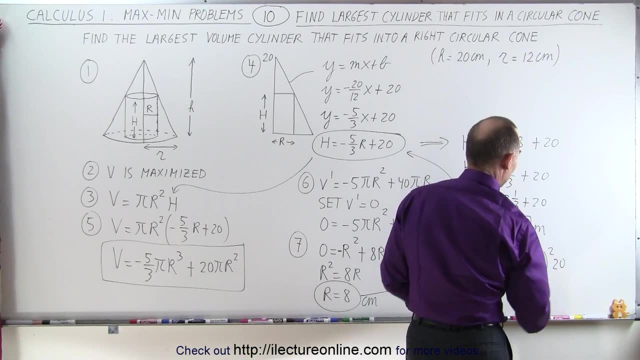 times the height, which is 20.. So approximate value of pi divided by 3 is approximately 1, 12 squared is 144, times 20, 288, that would be approximately 2880,, a little bit more because pi divided by 3. 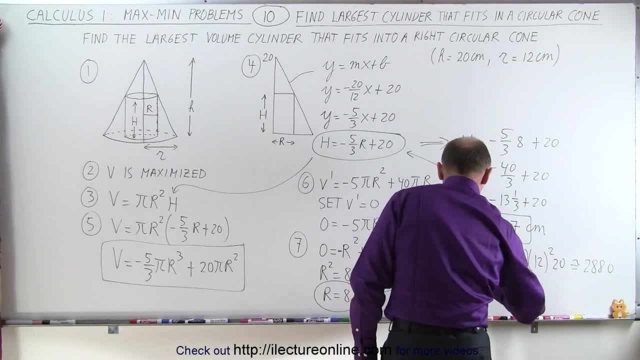 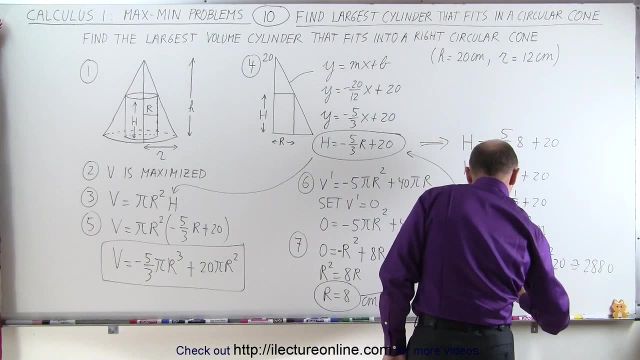 is a little bit more than 1.. And now let's find the volume of the cylinder And that would be area of the base times the height. so it would be: the area of the base would be pi times 8, squared times the height. 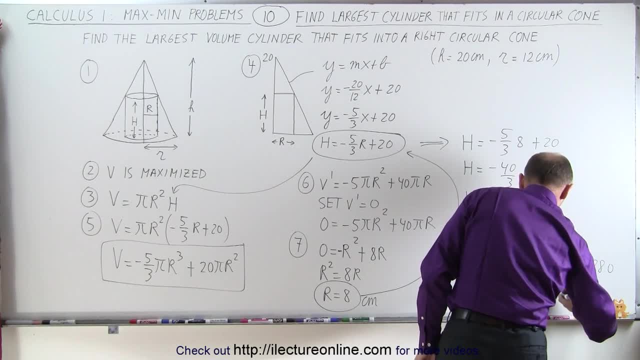 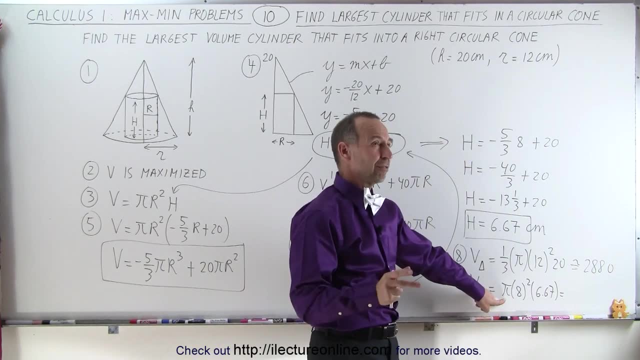 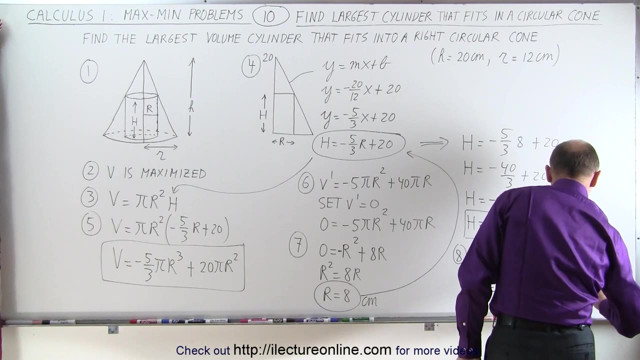 and the height was 6.67.. So again for approximate values, that would be 64 times pi, a little bit over 3, 64 times a little over 3 is about 200, times. this will give us about roughly 1350,. 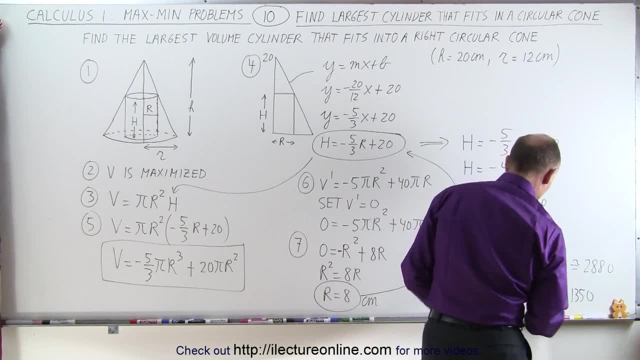 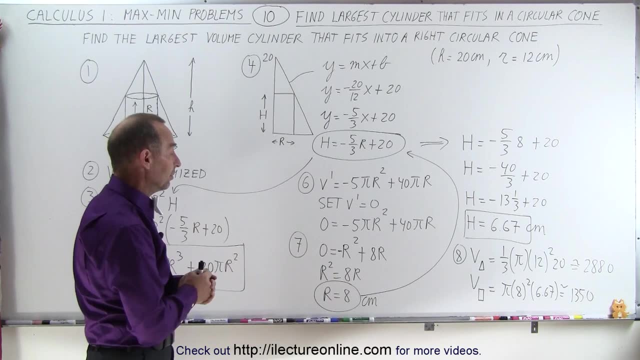 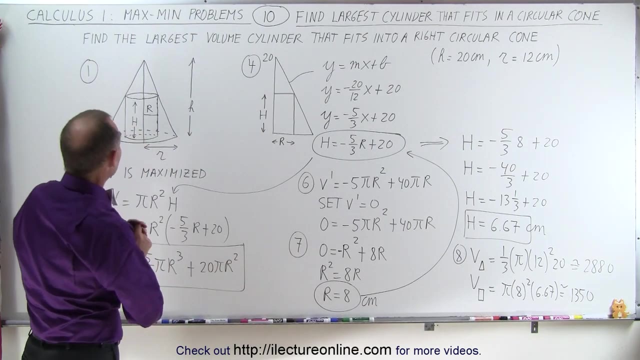 and you can see that that's roughly half of the volume of the right circular cone, which means that we can say that the values, at least, are reasonable. We don't know for sure it's correct, but we know that they are reasonable. Again, a quick review. 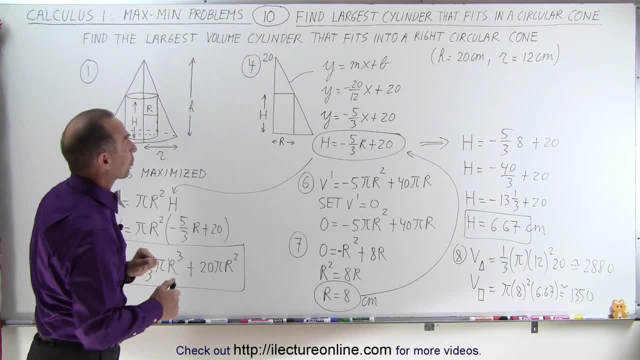 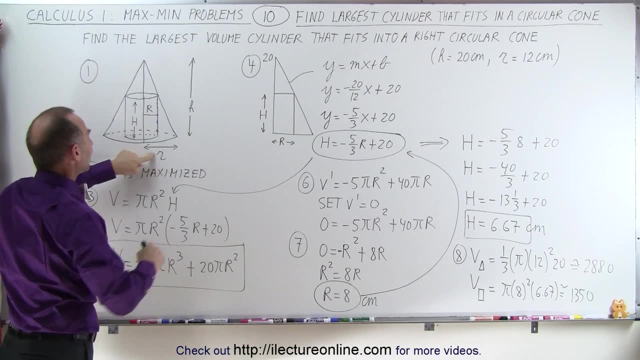 we're told to find the largest volume cylinder that fits into a right circular cone. We first start by drawing a diagram that shows the right circular cone and the cylinder. inside We label the variables for the right circular cone and the variables for the cylinder. 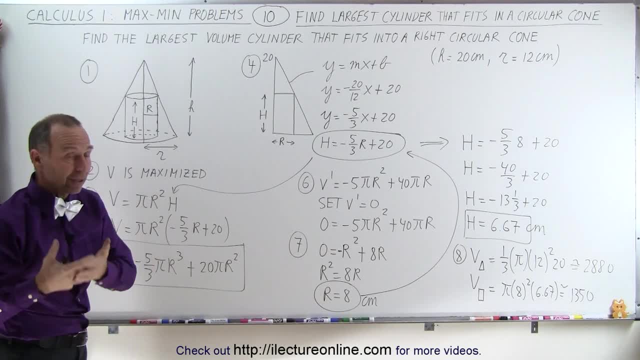 Step 2, we determine what's being maximized and we're trying to find the maximum volume of the cylinder. Then we come up with an equation: in terms of the unknown variables, The volume is the area of the base times the height. And then for step 4,, 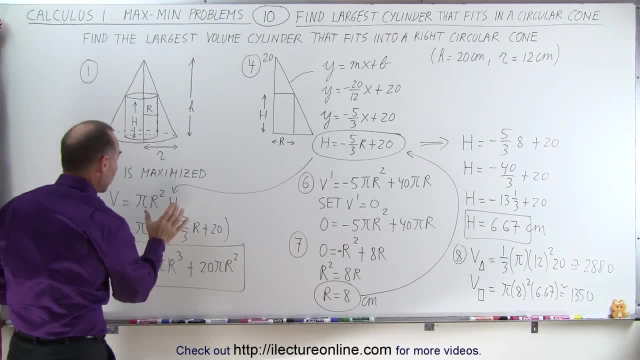 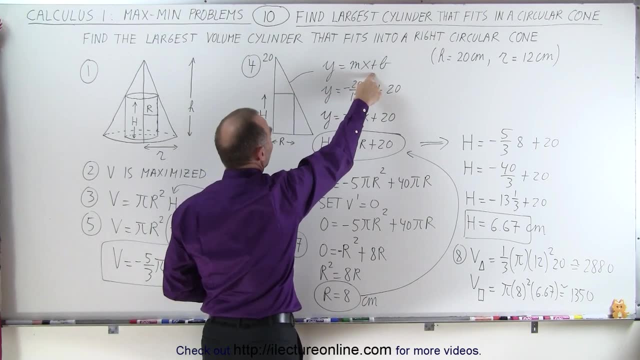 we try to find the constraint that will allow us to eliminate one of the variables And we use the concept of the straight line equation- y equals mx plus b- to relate the variables h and r of the cylinder to y and x of that straight line. 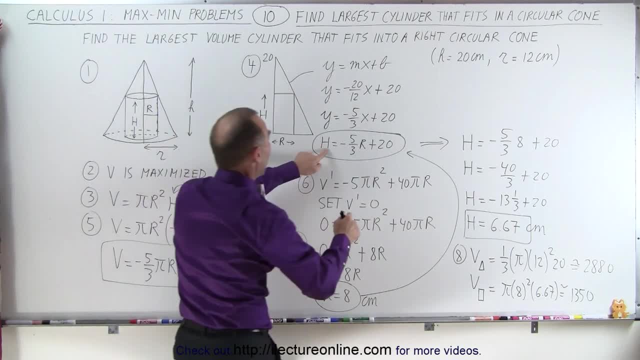 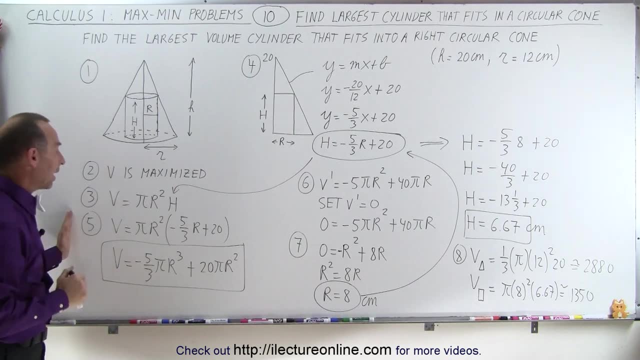 Once we've done that, we now have a relationship between the height and the radius of the cylinder- We solve for one of the variables and we eliminate h in this equation Now coming up an equation that is the volume, in terms of one variable only. 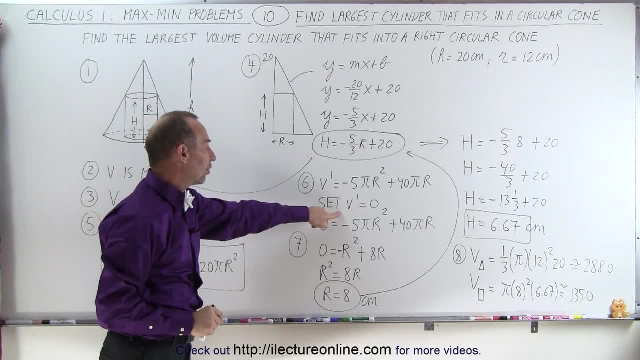 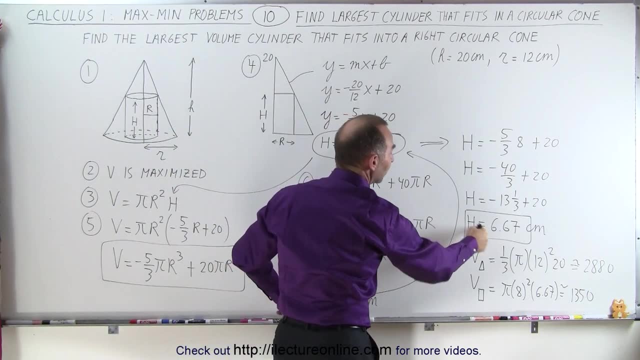 We then take the derivative of that, set it equal to zero, and then we solve for the unknown variable. Once we've done it for the one variable, we use a constraint, We get the value of the other variable and then we do a quick check. 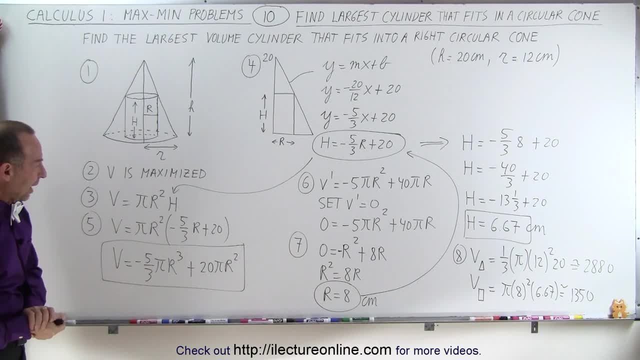 to make sure that we're in the ballpark, that it does seem to be correct And that's how it's done. 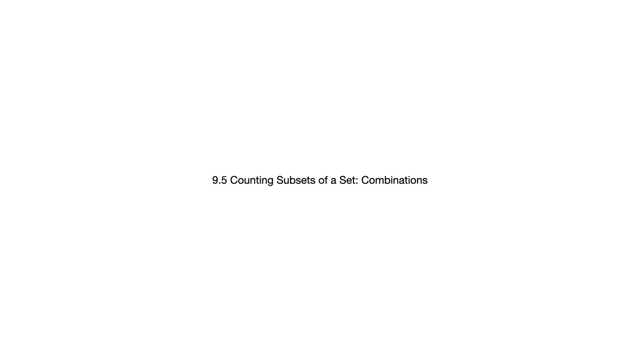 Let's have a look at section 9.5, counting subsets of a set, combinations. Now, combinations is a concept that we first saw in chapter 5, and we revisit it here in chapter 9, which makes sense, since chapter 9 has really been focused.